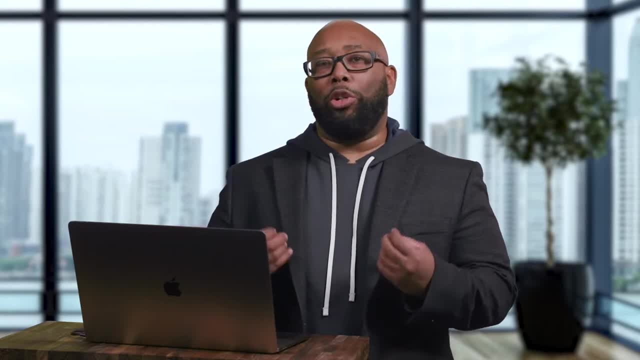 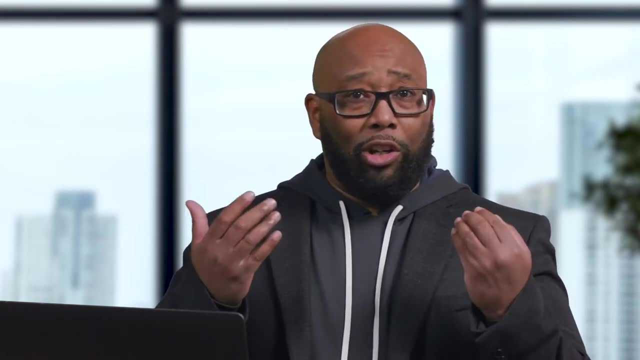 that are supposed to get us there. How do we measure how well we're doing Audits? Audits are how we figure out if we're meeting our requirements, whether or not we have the controls in place to even measure or assess whether we're being secure or moving towards security. 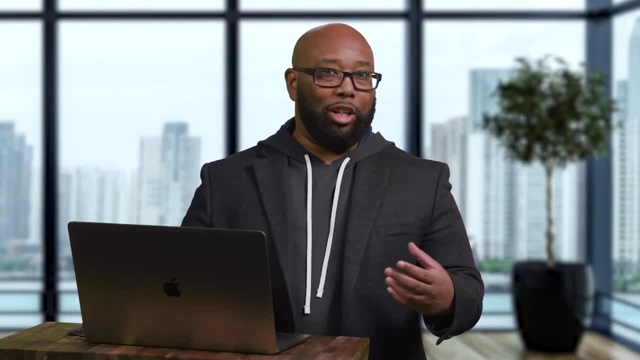 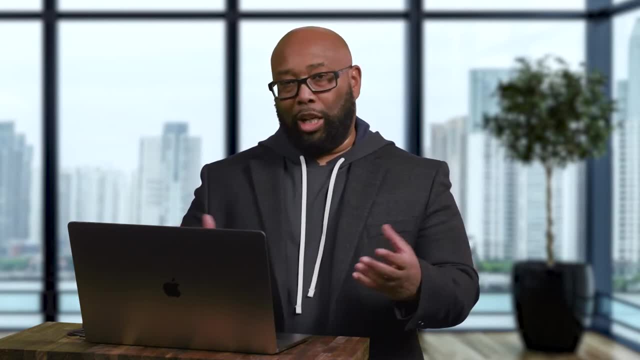 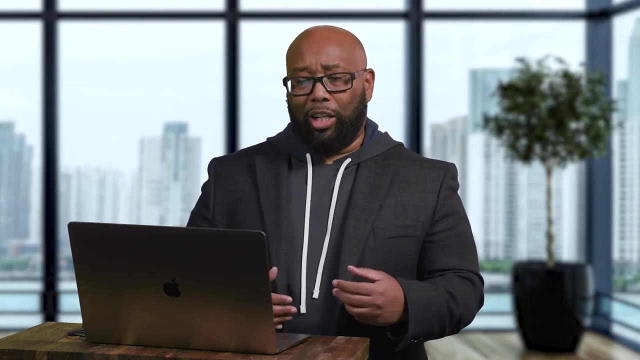 This is one of the areas that again, to me, is one of the unsung hero types of roles in cybersecurity, because it does not necessarily get the glamour, the exposure and all the other things that some of the other sexier roles in cybersecurity get. But let's talk about audit and what it means in 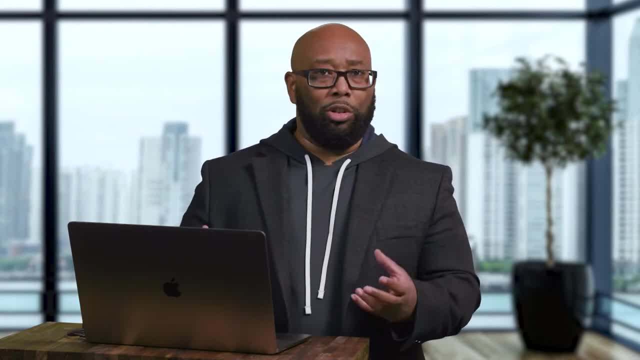 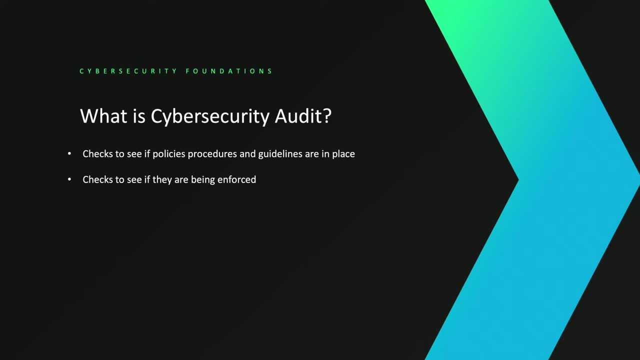 the world of cybersecurity and exactly what the auditors do and how. they're an invaluable part of what we do in cybersecurity. What is cybersecurity audit? Well, we're checking to see if policies, procedures and guidelines are actually in place. Then we're also checking to 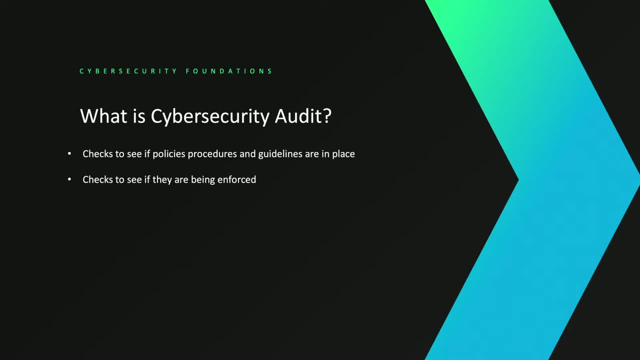 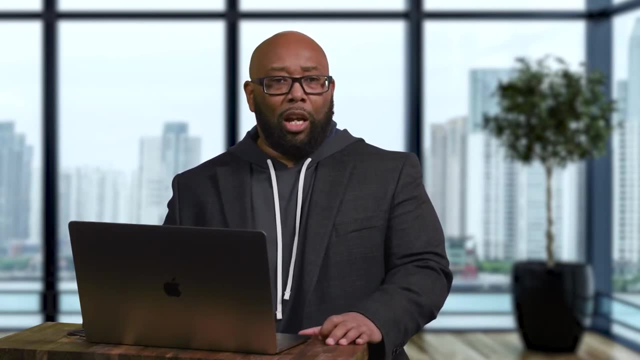 see if they're being enforced. Then, further, how are you enforcing them? Because here's the thing. here's what I found out from being in cybersecurity. One of the things that I get called on to do regularly is I have a lot of people that I've mentored that went on to be 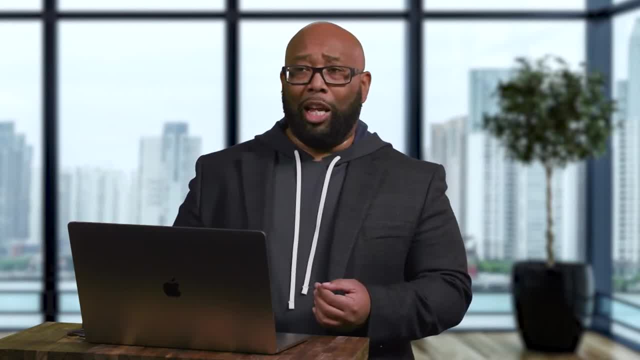 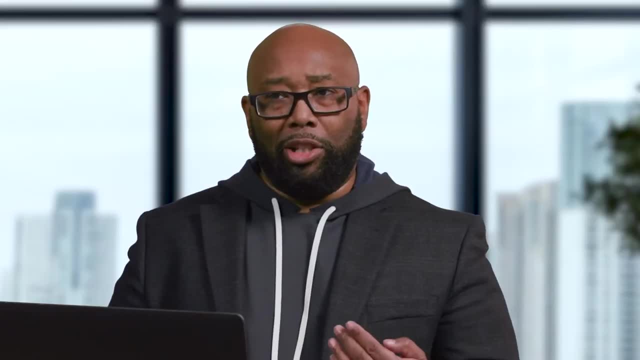 security auditors. They didn't go the technical route like me, to become a pen tester or a threat hunter or an incident response person. They went the audit route On a regular basis. some enterprise organizations audit practice will bring in people like me to help them audit. 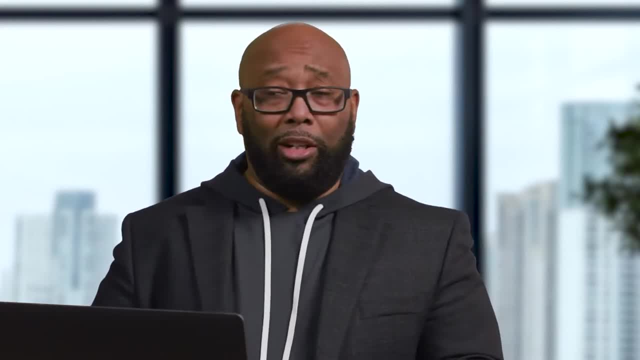 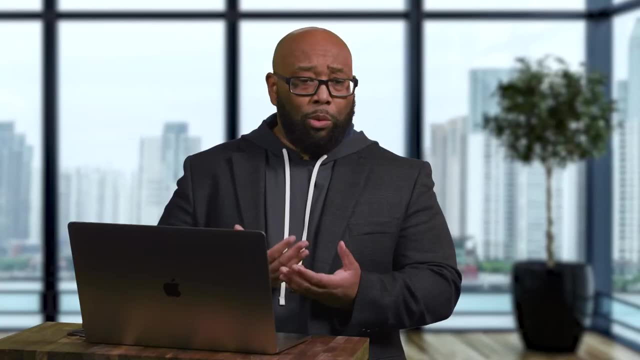 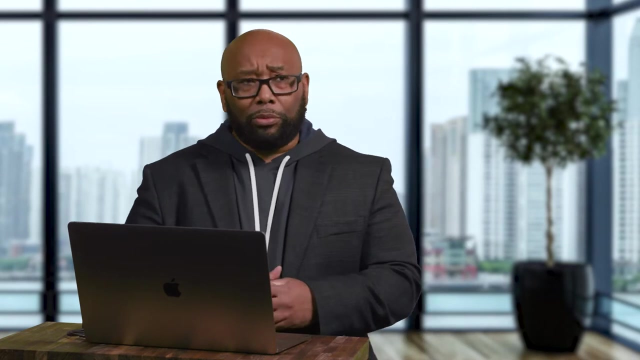 a cybersecurity team's cybersecurity practice. It could be anything from incident response to how they do pen testing to how they do vulnerability management. whatever the case may be, The number one thing that we find when we go out and assist the actual cybersecurity auditors in these audits is that most organizations have 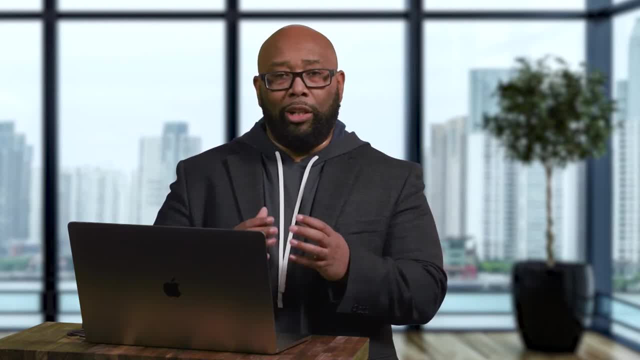 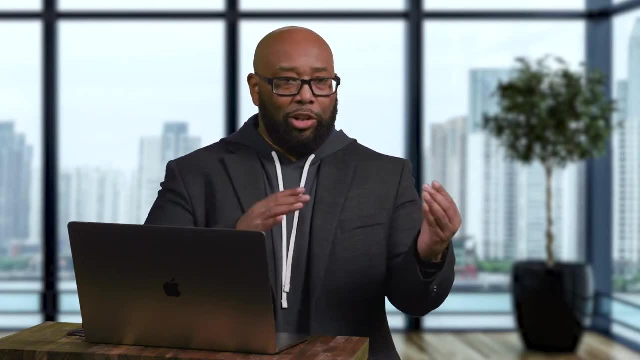 policies that on paper, these things read like a Stephen King novel, like they're perfect policies. It's like good stuff, like these things. they're doing this and they have this in place and they're always checking this and they check this and they do this every day. 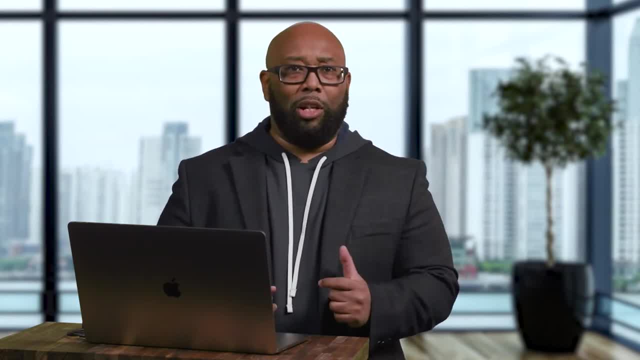 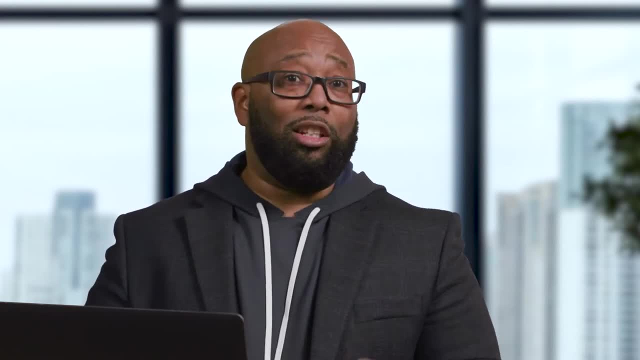 And every 30 days they roll this out and they check it this way and they double check it that way. Looking at that paper, looking at that policy, everything looks great. Now, when you start doing actual auditing and you say: great, these things are awesome. 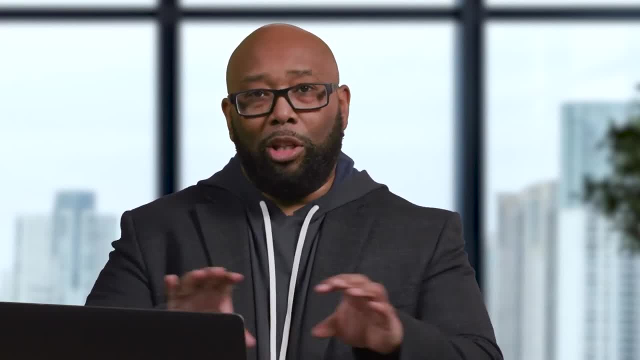 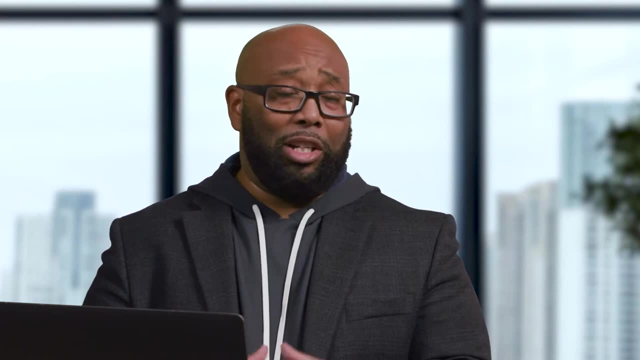 Nobody else has it this well refined. You start pulling back the layers and saying, OK, well, we want to audit how you're doing this and we want to watch it and see what's actually happening, And then it starts to fall apart in a lot of cases. 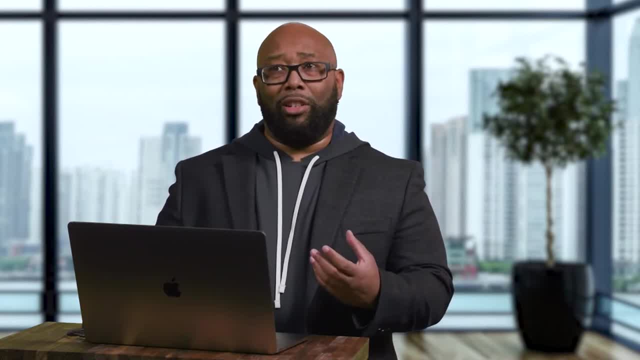 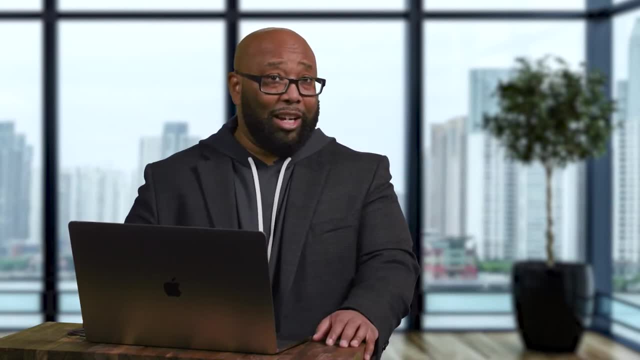 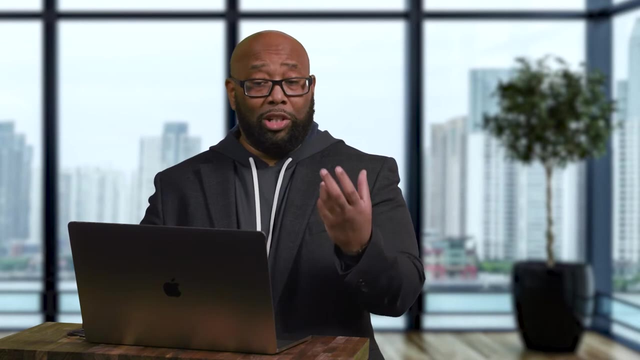 So what ends up happening is we find that about half the things that they have written in their policies or procedure documents they're just not doing When they're actually doing everyday operations. And these are some of the things that we uncover, And this is one of the, this is one of the reasons audit is so, so valuable. 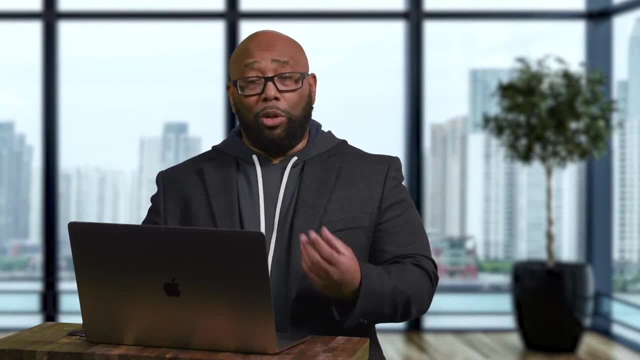 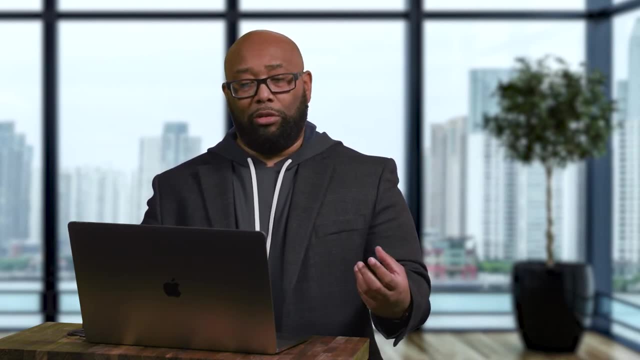 So, if you decide to go this route and become an auditor, those are the types of things you'll be doing. You'll be looking at policies, looking at statements and then asking the questions: How are you doing this? Why are you doing it? What does it mean? 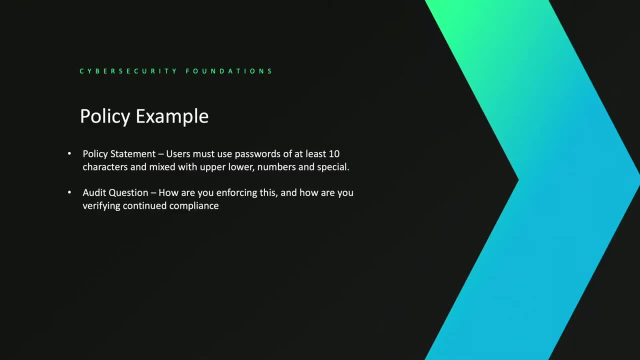 So let's look at some other examples here. So here's a policy example. You have a policy, You have a policy statement that says users must use passwords of at least 10 characters and they should be mixed with upper and lower numbers and special characters. 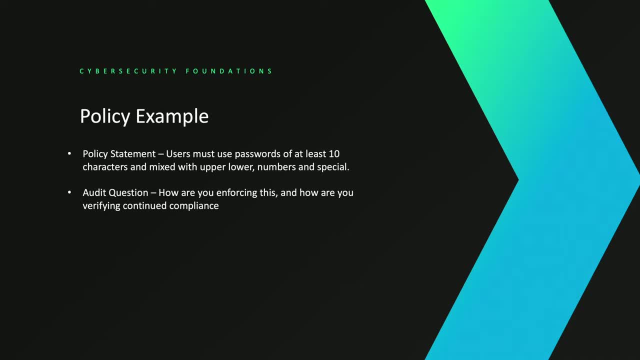 Well, an audit question would be great. You have this policy that says that: How are you enforcing this and how are you verifying continued compliance? Now, when you look at that cyber security or an IT security team should be able to come, 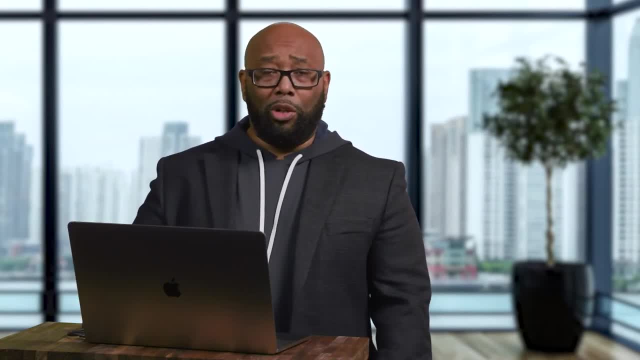 back and say is: oh well, we enforce it because we roll out something called a group policy that won't allow a user to create a password that's less than 10 characters and doesn't meet this criteria. So at the technical level, we have a technical control which is: 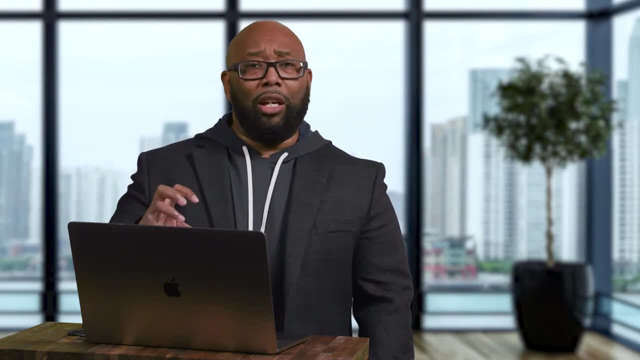 another big audit term control. We have a technical control that forces them to use a strong password or else they won't be able to create their account or create their password. So we're enforcing it that way And we're verifying continued compliance, because we do our own. 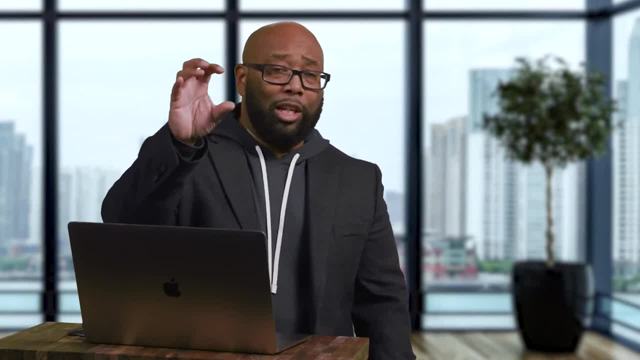 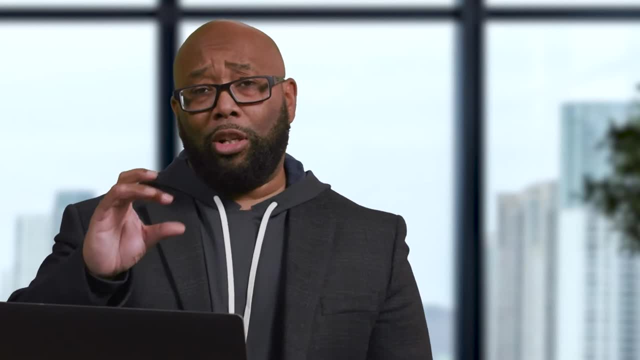 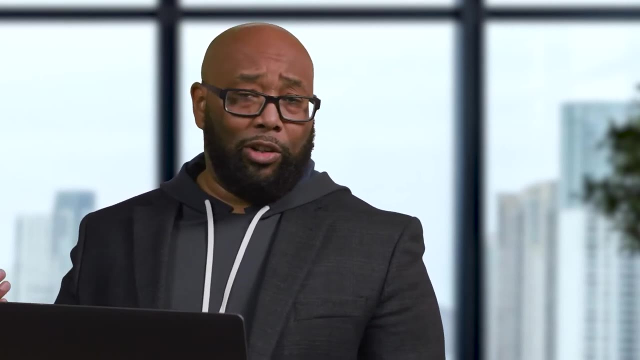 password audits. every month We will take a sampling of 10 percent of our user base and we will run password crackers just like a hacker would. We run password crackers against their password hashes to see if we're able to crack them in a reasonable amount of time, And we also check to see how many of them are actually. 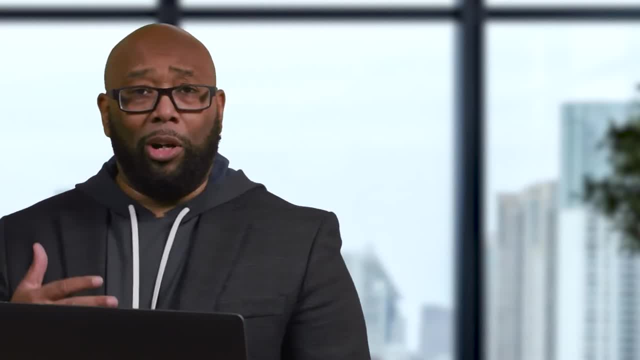 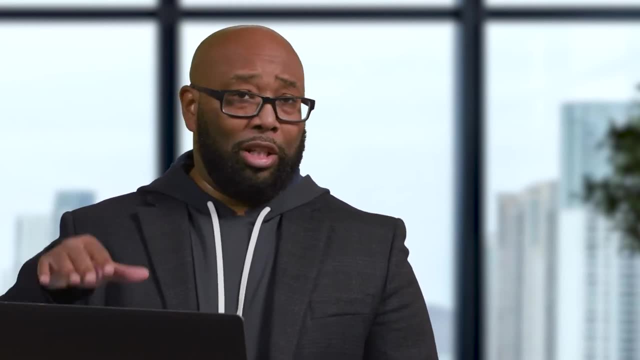 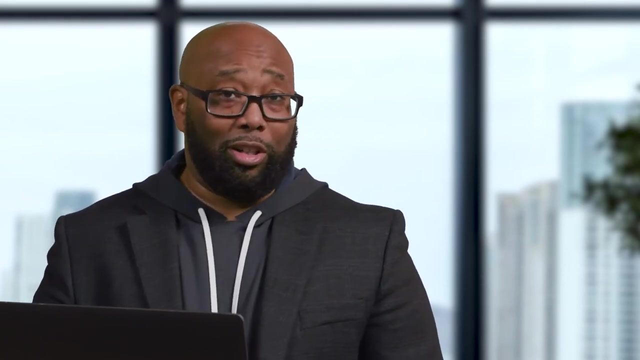 strong passwords. So that would be a valid response. Now, as an auditor, you want to hear those things because it shows that they're actually validating the controls that they've put into place. But if you go and audit and you start, You know, hearing, they give you more paperwork when you ask for paperwork and it says we do A, B and C 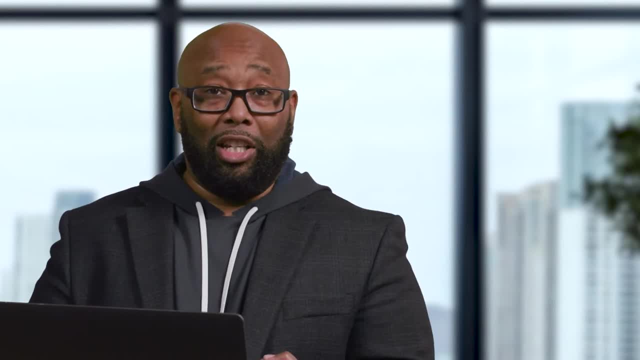 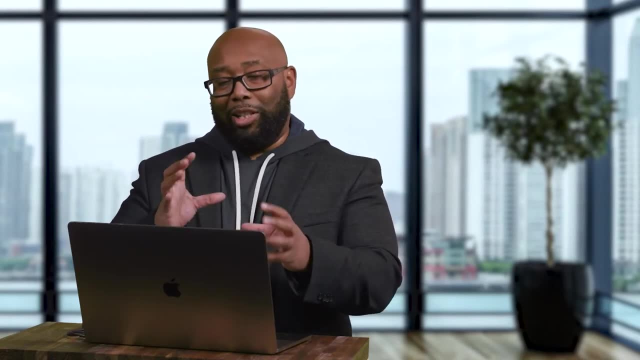 and then you say, all right, well, how are you validating it If they just give you more paperwork that says: you know, we validate it by saying this on paper? that's not the same thing. So this is a classic example of what you might run into if you end up being an auditor. 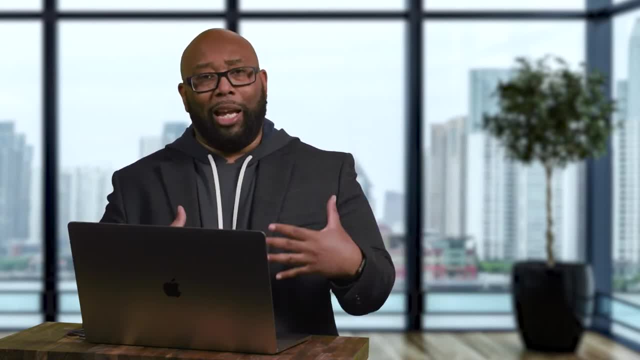 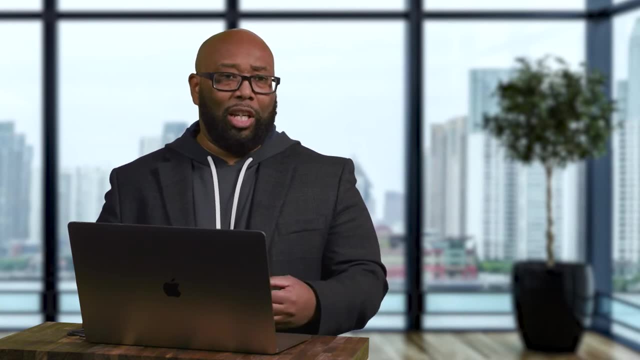 Now here's where I want to tie this entire learning path together. Think about what I just said there. If you didn't understand what a password crack is or what hashing is, you may not, as an auditor, understand the relevance of what I just said. 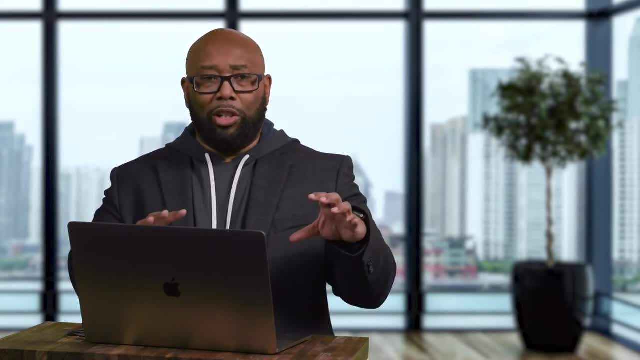 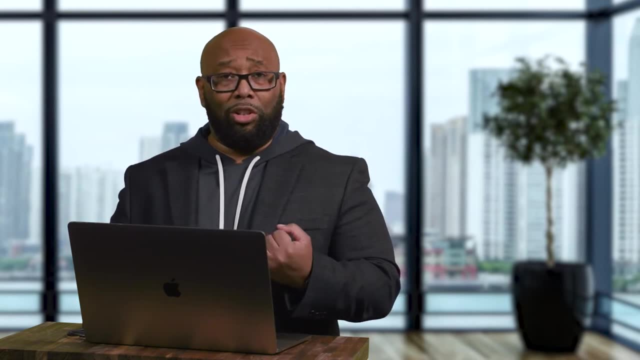 So this is why this course is meant to be very, very ground level, to kind of give everybody a touch of everything, because auditors do need to know and understand what password cracking is, you know what a strong password is and what group policy is. 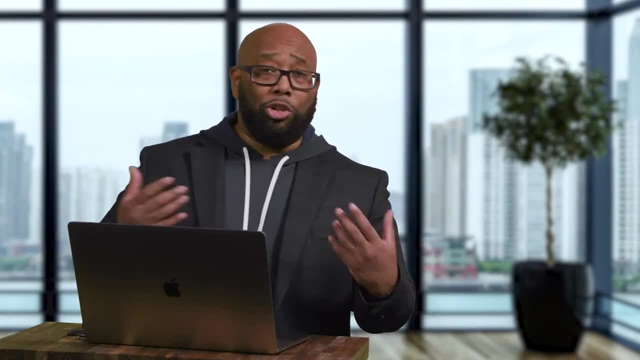 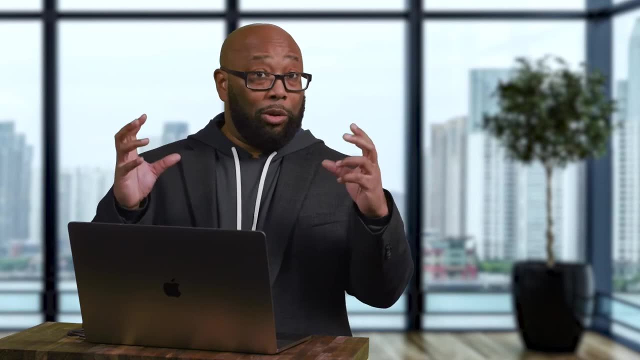 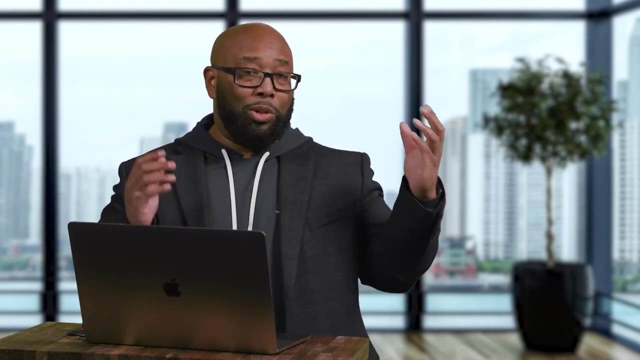 I just passively said we roll out group policy to ensure that they can't create weak passwords. Well, if you don't, you don't know that group policy is something where you can go into Active Directory, which is a Windows domain management database, and set a rule one place that says no passwords less than 10 characters. 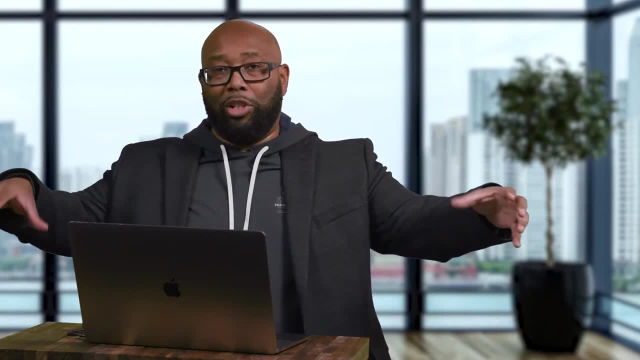 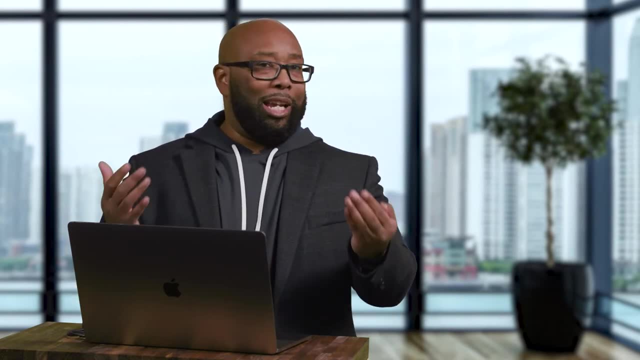 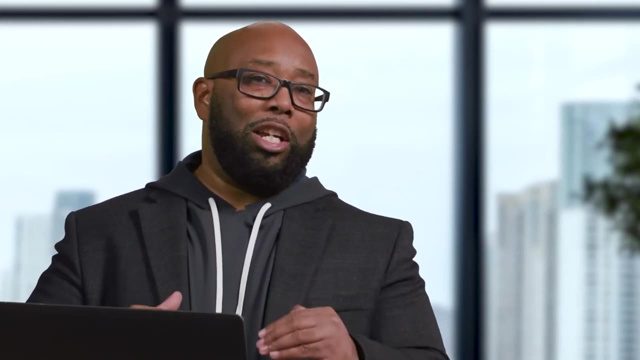 And then that rule automatically rolls out to everyone in that organization. that's part of that domain. If you didn't understand that, then when I passively said we have a group policy object that does it, it wouldn't make sense to you, And this is one of the main things that I've stressed since the beginning of this course- is having that foundational. 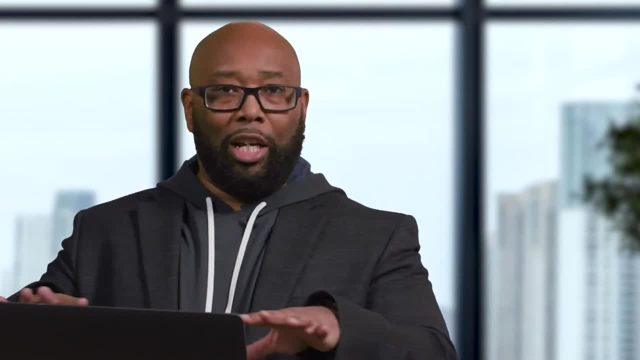 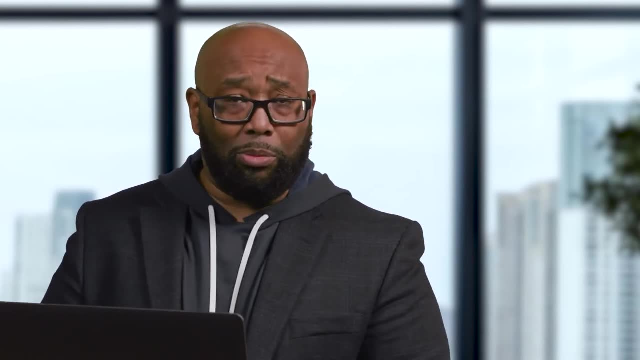 foundational knowledge, understand the operating systems that are underneath everything else, because then you can understand where these controls actually come in and how they work. And this is just one example. Now let's move on and look at another example. Let's look at a procedures example. 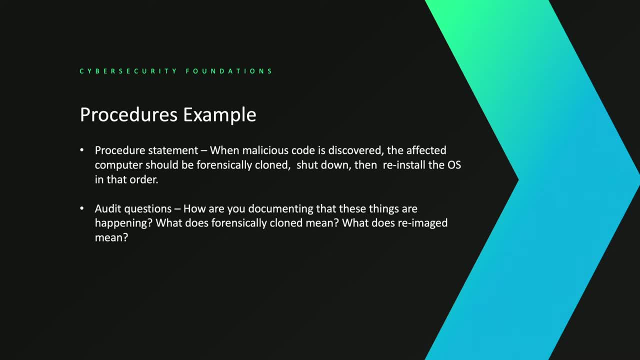 You might have a procedural statement that says: when malicious code is discovered, the effect that computers should be forensically cloned, shut down, then reinstall the operating system in that order. An auditor would see that and start ripping it apart by saying, well, yeah, this sounds great. 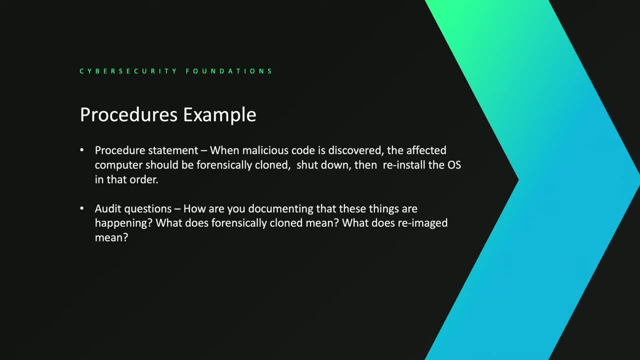 But questions are: how are you documenting that these things are happening? Are you actually doing them, or is it just something you have in policy? Secondly, they might come back and say: well, you can't just throw blanket open ended terms out there like forensically cloned. 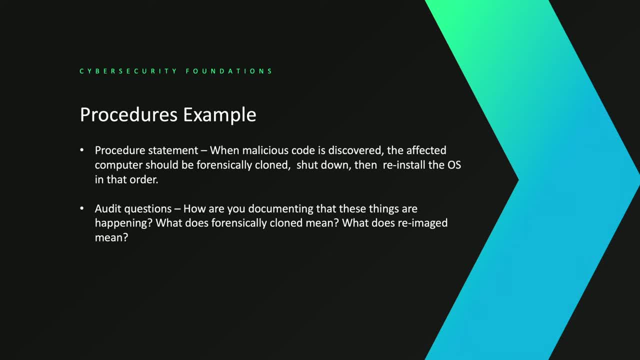 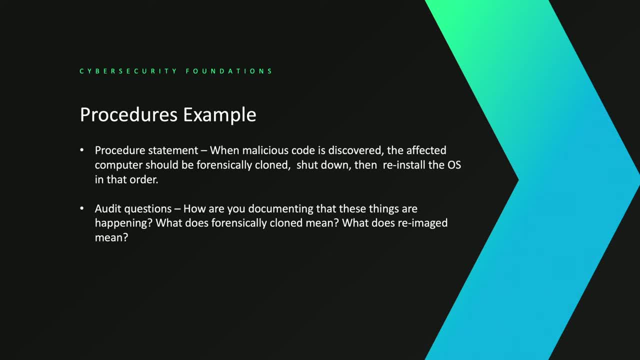 But for organization B, forensically cloned might mean something else, But for organization A forensically cloned might mean something totally different. So for that, control the forensically cloned. what do you mean by that? We need something definitive, because how are we going to check to see if you do it? 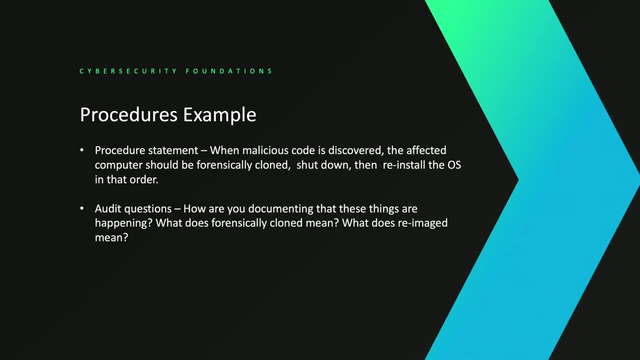 And if we don't even have a you know metrics to know what that is, then they might come back and say: and what does reimage mean, you know? or what does reinstall mean? Because if you're saying you're reinstalling the OS, I got news for you. 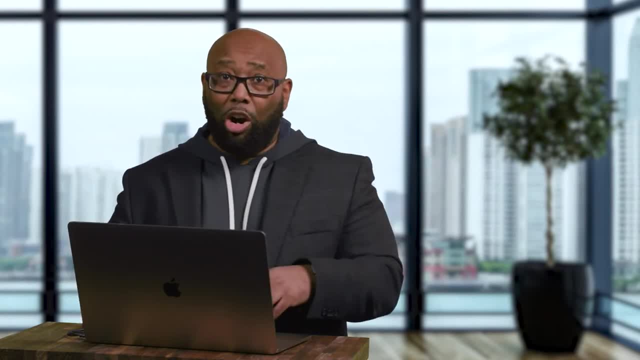 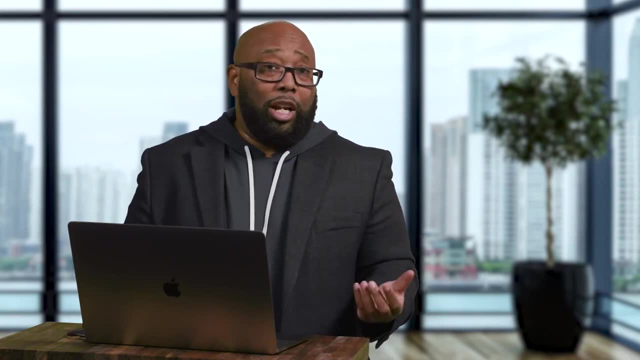 Most of the modern kernel level, or you know, some of the hardware root kits that are out there now. doing a reinstall of Windows does nothing to get rid of that malware. It's still there. When you reinstall Windows, you just have a clean install of Windows that's also now infected with malware. 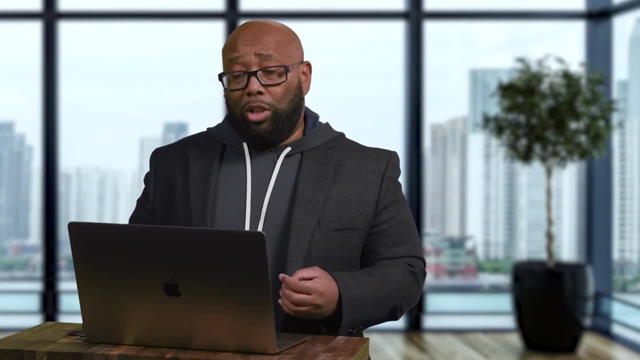 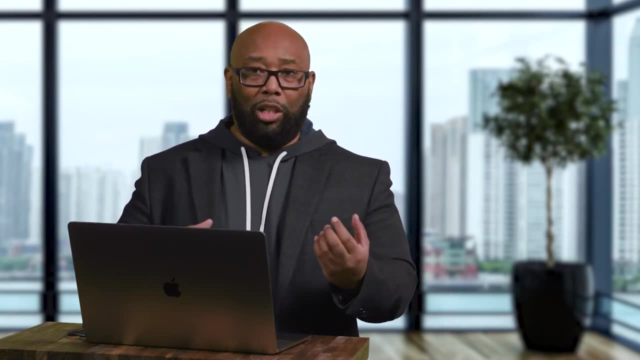 So what good did you do? Really none. Now, if you say re-imaged, which is what we're saying in the audit question, then that means something totally different. It means that you took that machine and you completely re-imaged it. 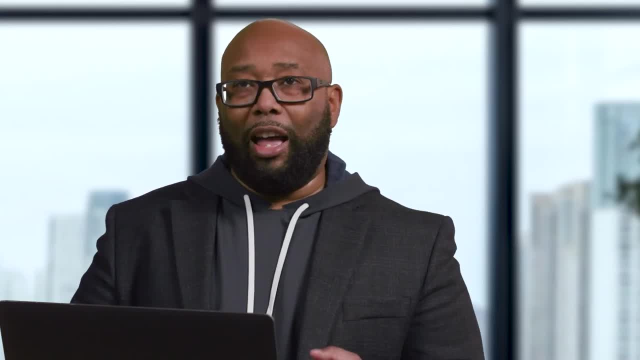 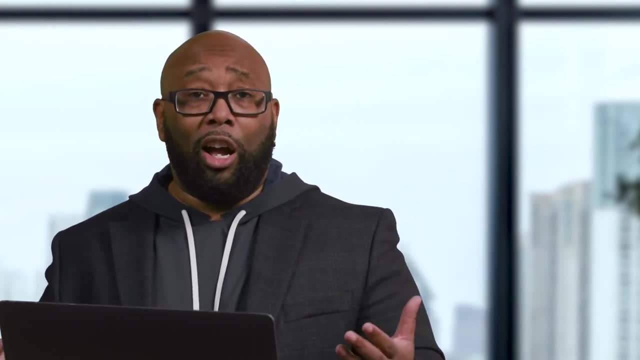 It's not the same as just doing a reinstall. So you have to make sure you define what these things actually mean. So you have to make sure you define what these things actually mean. Now I've actually run into a situation to where we were working on an audit. 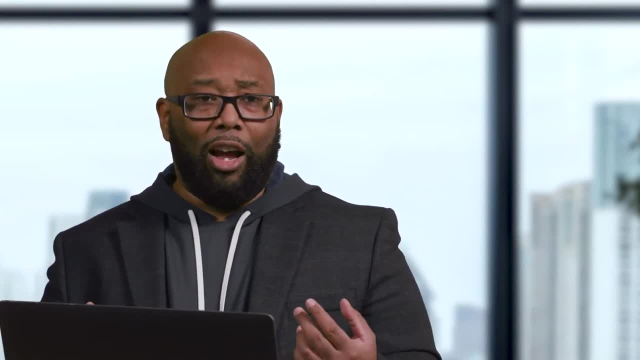 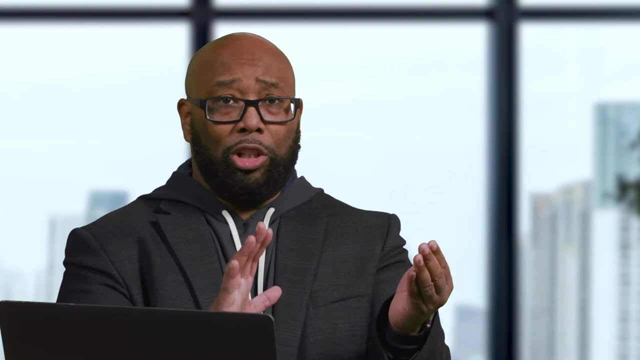 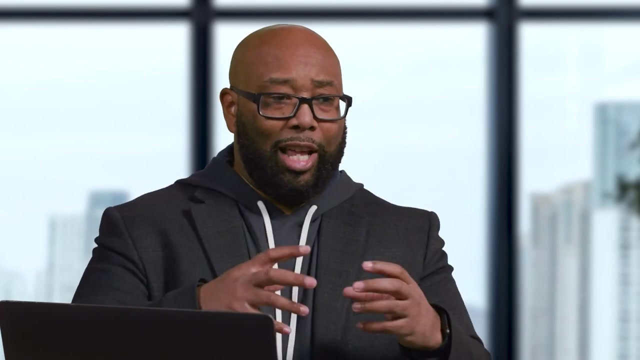 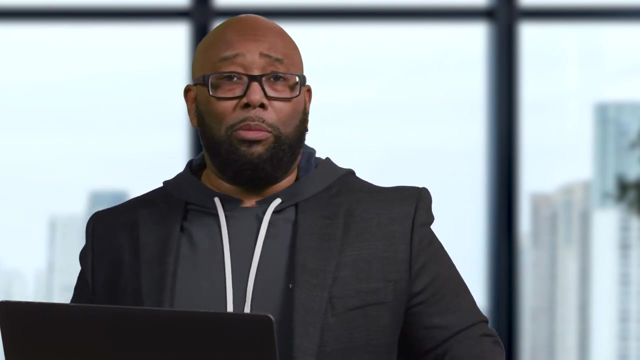 I was assisting an audit team where they were looking at how a big organization was responding to infected devices And really what you had was you had the cybersecurity team that would identify these devices that are infected with malware, And then they would kind of take that responsibility, wrap it in the paper and throw it across the wall to the IT team and say, look, we don't do images. 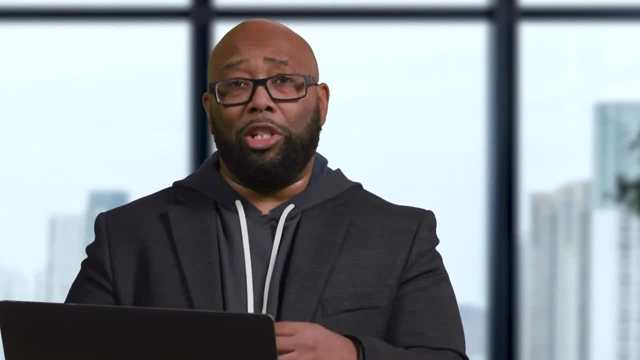 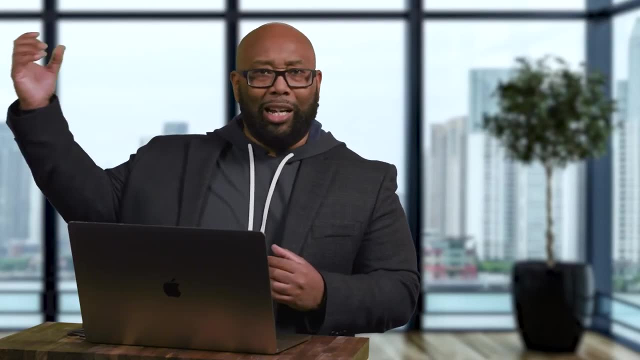 We don't do re-imaging, We don't have anything to do with the company images And, by the way, an image is like a snapshot, right? If your computer breaks or you get a new computer they can pull out of, like a database, a snapshot of your exact computer configuration- it was the day you got it- and push that out. 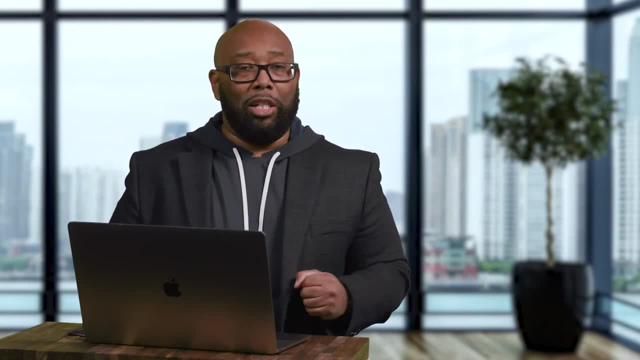 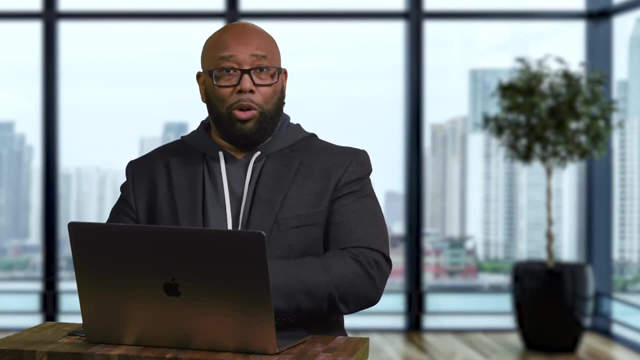 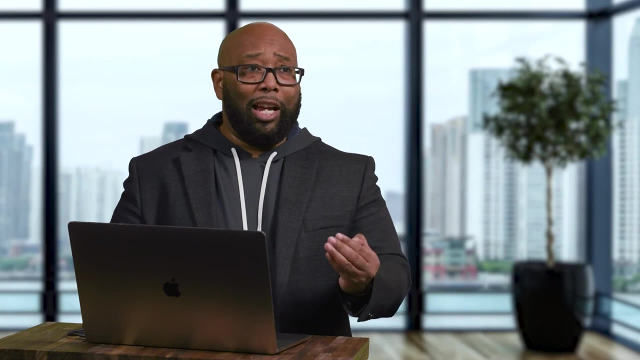 And your computer is magically back how it was then. And this is how we operate in IT And generally that's an IT responsibility from a day-to-day operation standpoint. But what we found out in that audit Was like: look you cybersecurity people you need to define to IT what you mean by audit. 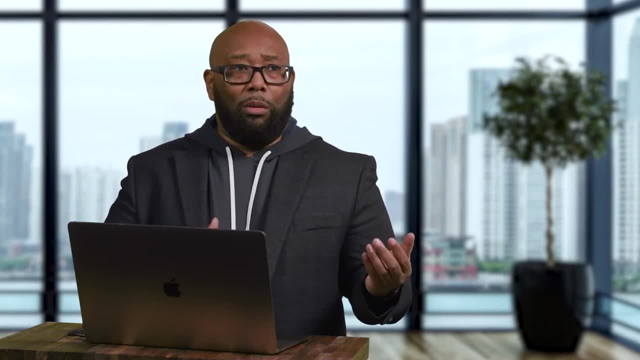 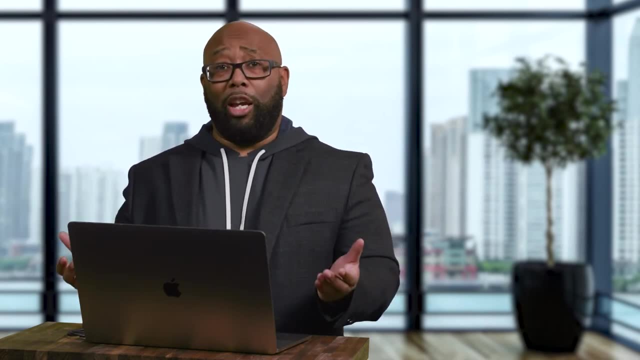 Because the fact of the matter- or excuse me what you mean by reinstall or re-image- Because the fact of the matter is: re-imaging it may be okay, Re-installing is absolutely not okay, Because you didn't really do anything. 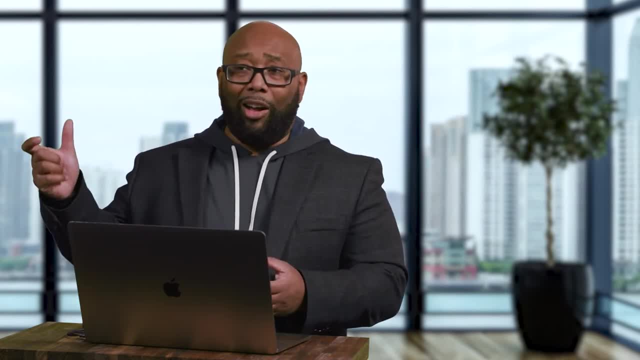 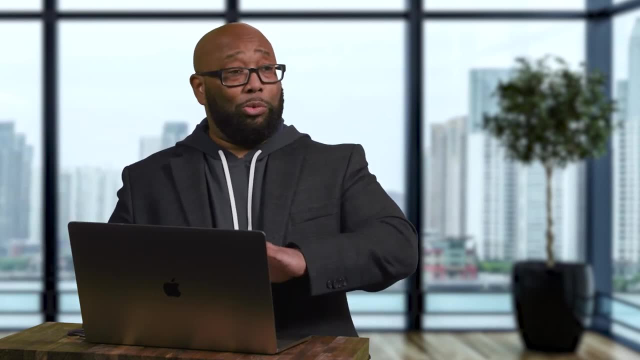 So you might have given that role to IT. But now IT reinstalls Windows on that machine, Pushes it back into production on the enterprise network And just reinfected The network after you've went through your whole expensive incident response eradication process. 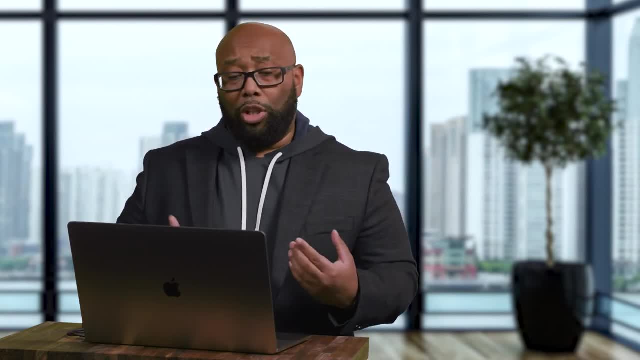 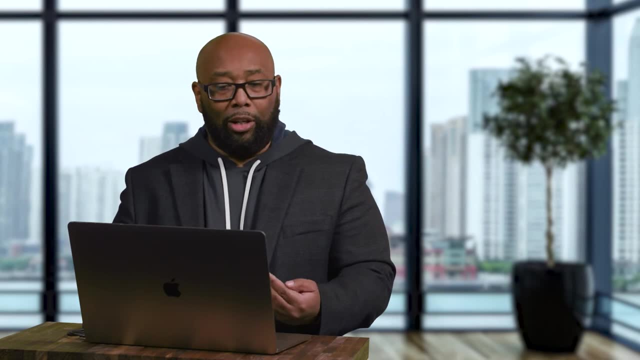 Now you just reinfected everything, right? So this is the types of questions you, as an auditor, can come and look at. You might say: well, you know, I think you need to better define what you mean by reinstall. Maybe you should be re-imaging. 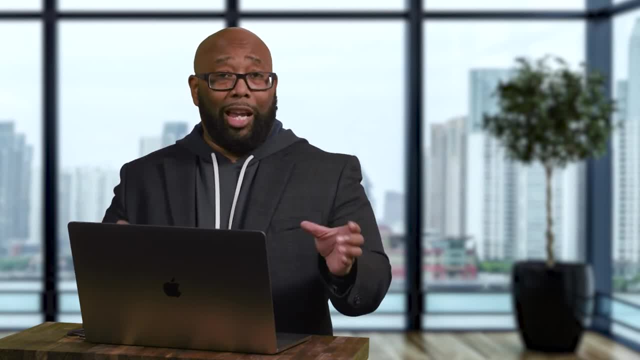 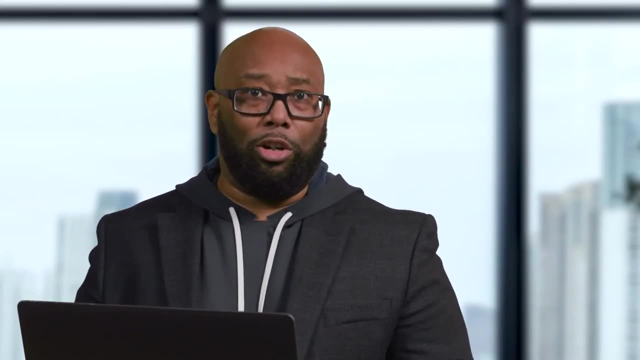 And if you're re-imaging and you said reinstall, you should phrase it as re-image, Because it means something completely different. And when you hear people in cybersecurity and IT complain about auditors being picky, it's not that auditors are being picky. 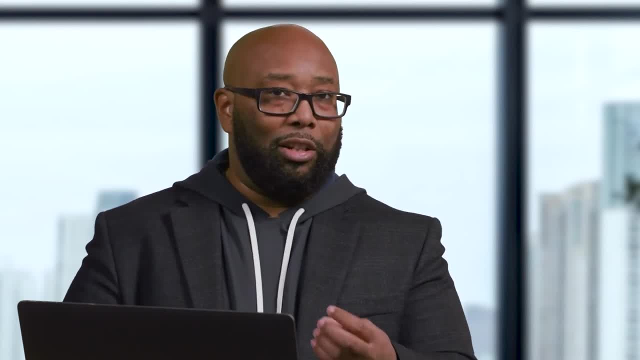 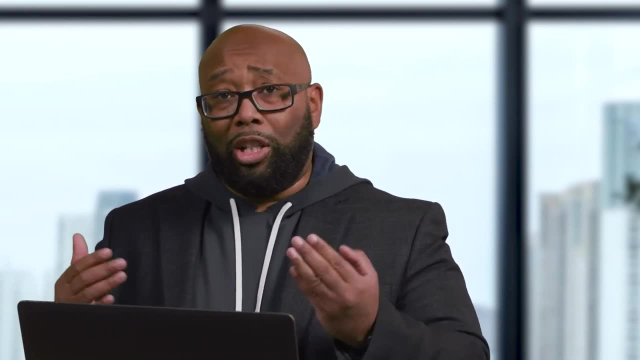 It's because difference in words and different phrasing and the way that you state these things, it absolutely has material difference in what you end up with. So it's their job to be that way, because it's necessary for them to be that way.